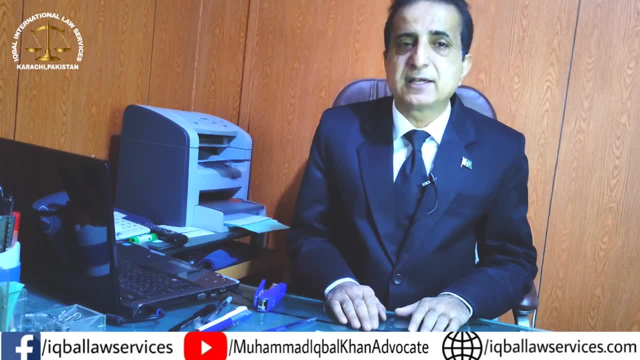 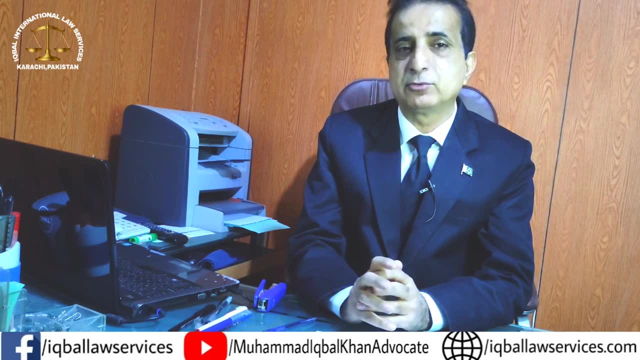 They will be paid. The corresponding course and fees will be paid. The documents will be prepared. Both parties will appear before the registrar of the property. He will take his statement and after that he will take his sign and thumb impression To be registered. 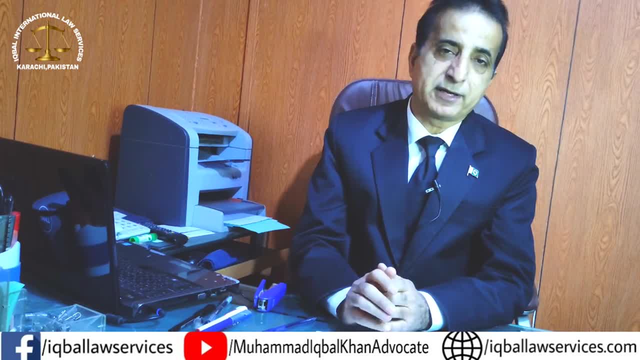 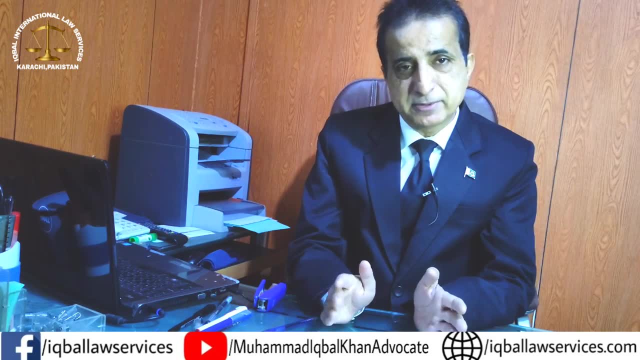 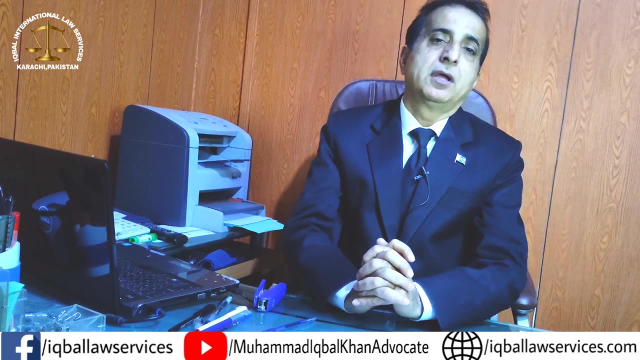 The documents will also be submitted to the registrar. The registrar will accept the consideration That of course I sold the property and I have handed over the property After that. when these documents are registered, the next procedure is mutation. You understand that the mutaish is such a thing that the name of the taxpayer is to be changed. 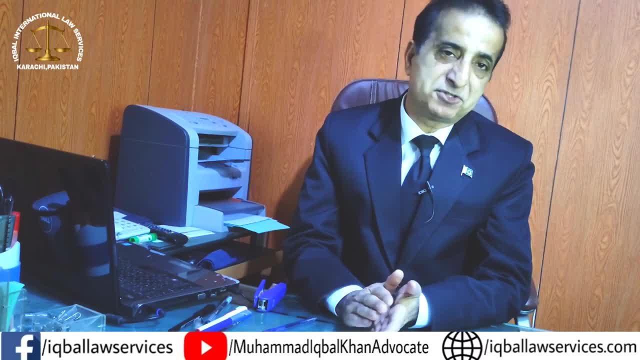 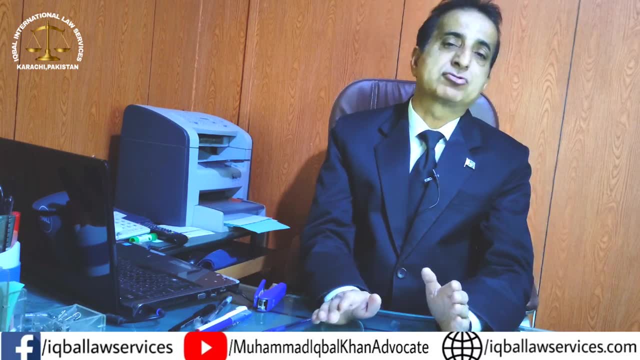 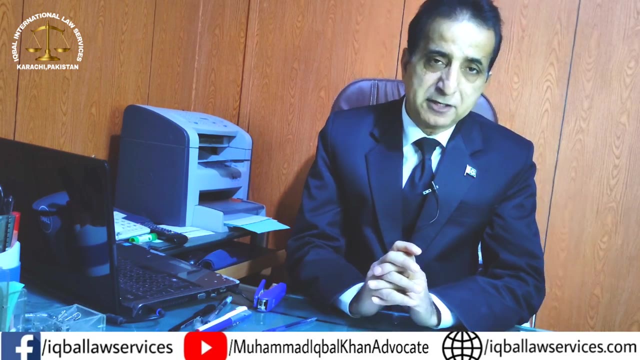 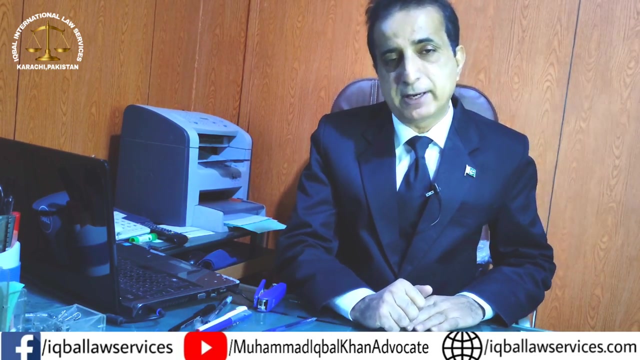 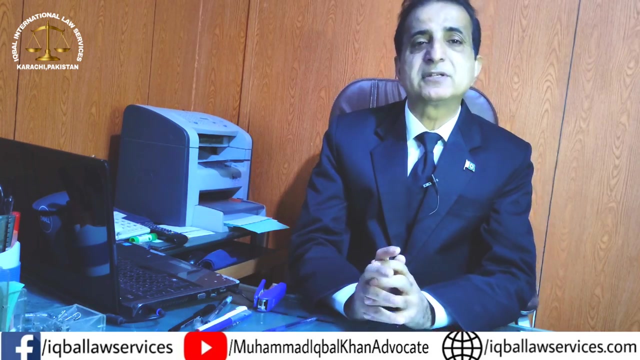 In the government department the name of taxpayer is changed. That means the right record in one owner to the other is to be changed. Go to the owner so that he can get help in the tax payer. the government tax payer is the change of one person to another person. this is called mutation, ie change in the record of rights. now change in the record of rights. it will be called mutation, ie mutation will happen after registration. when registration will be reversed, then it will be the turn of mutation. so after that mutation will happen. mutation will happen in the municipal record. in the government record of rights in the revenue department the title will change. 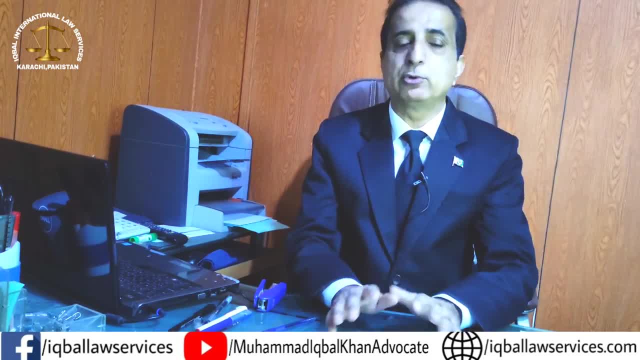 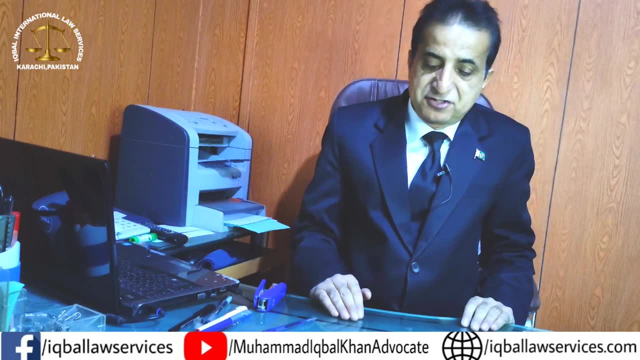 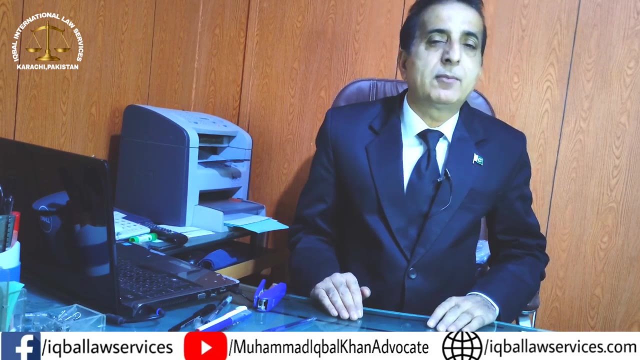 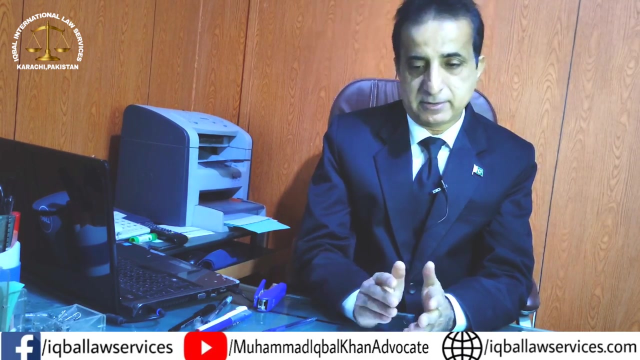 the new owner who bought the property will be called mutation. now, registration transfer is a legal transfer. registration will be transferred, whereas mutation will happen in the personal department. now the question is that whether we will sell this property without mutation property. now we do not have time and, due to lack of time, we want to buy the property now we need it. so why don't we sell this property? 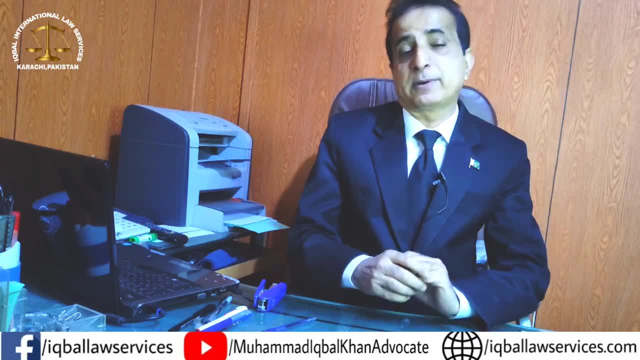 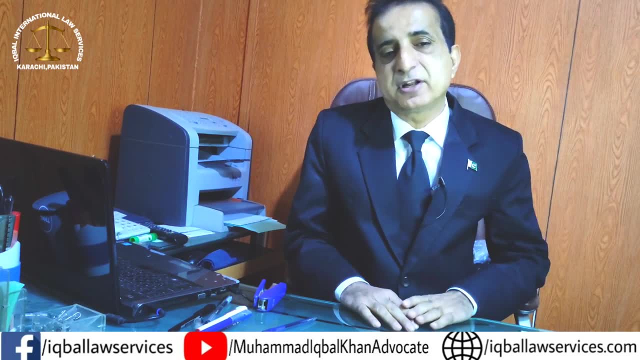 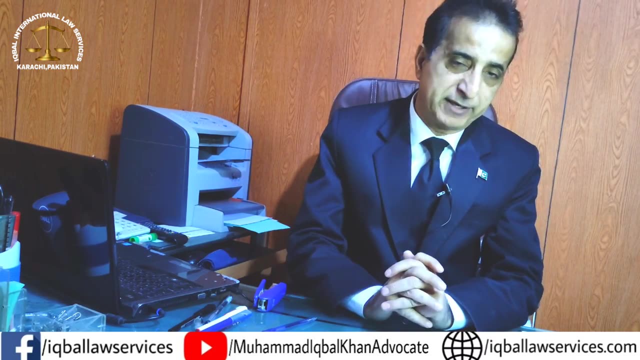 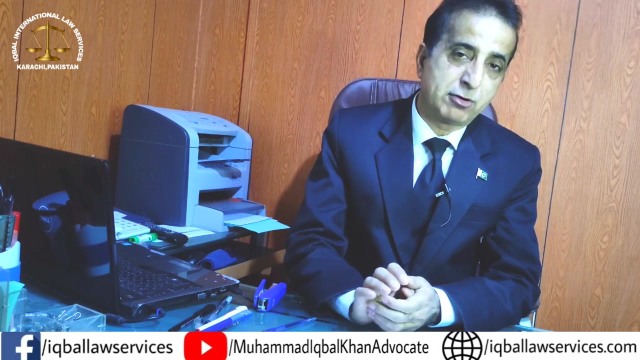 so basically, what happens is that we have already made a mutation of that property. if we do not make a mutation- we are in a hurry- then at that time we can sell that property directly on the registration document. the next registration document will be made to sell it, but it will be better- many objections can also be made- that you make a mutation and bring it, because it is necessary to change in the record of rights as well.